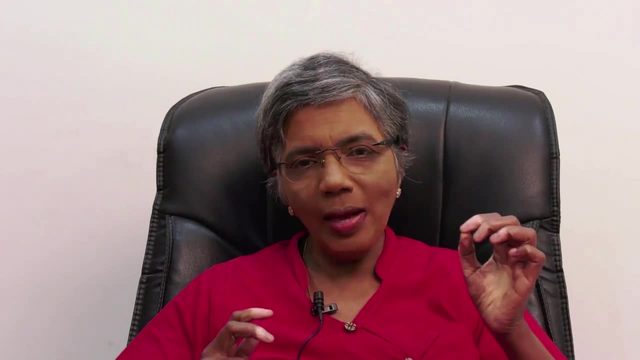 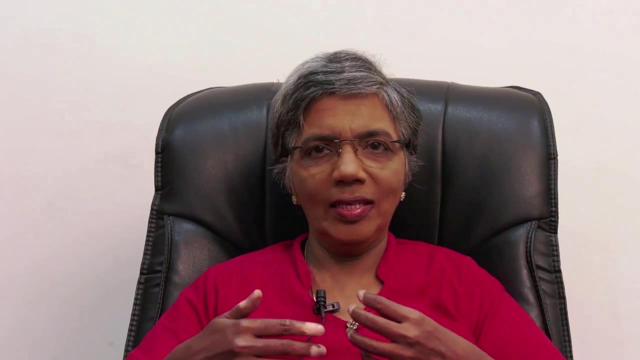 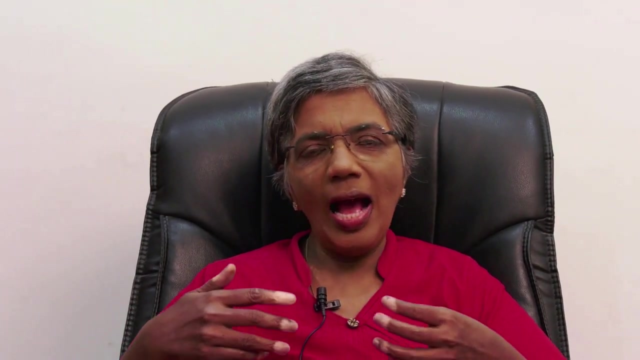 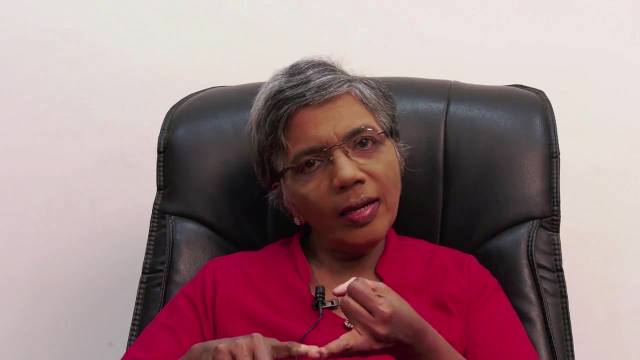 observe a smaller kid. more or less they wake up at the same time. They eat at the same time. Having this as a base, train your child. Start with the basic thing of food. Have your breakfast sometime- It could be seven o'clock or eight o'clock- Then their lunch at one time, Snack at the same time. 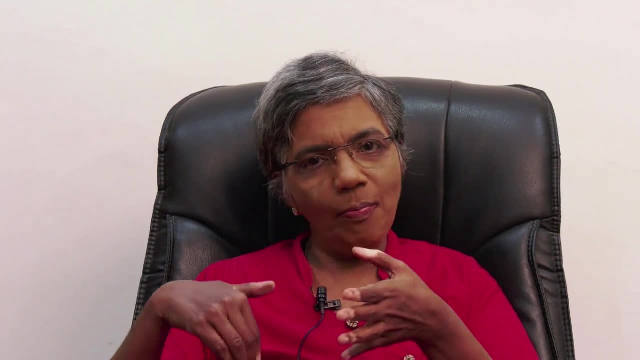 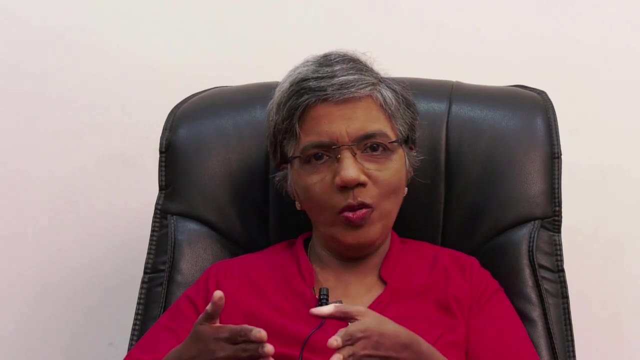 And dinner at the same time, With this as a base form their work. So, after breakfast, what do they do? For an hour, what do they do? And after that, the next hour, what do they do? It can be divided. 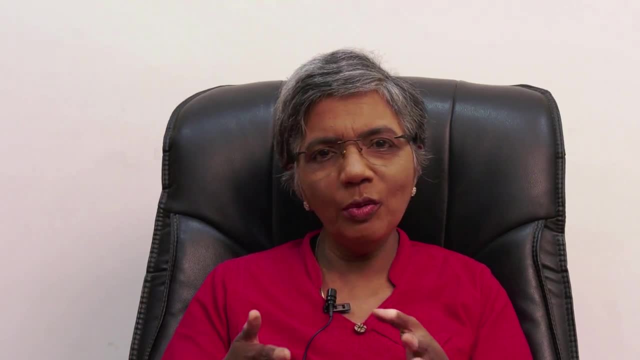 between these meals And if you do that, then I think a second time you will be able to do a lot of things. And if you do that, then I think a second time you will be able to do a lot of things. And 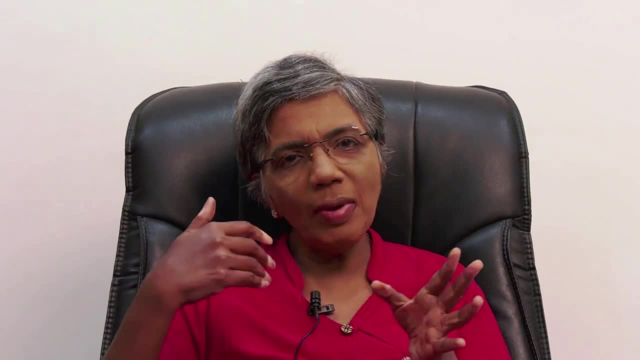 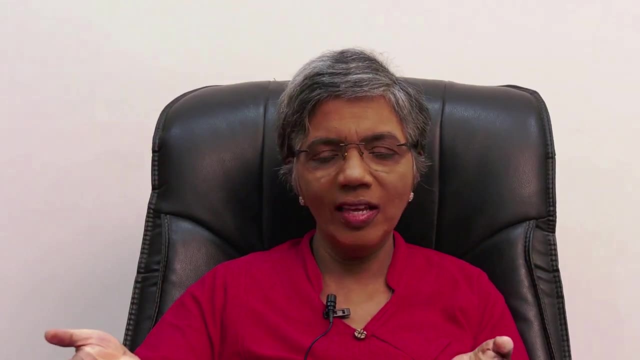 if you do that, then I think a second time you will be able to do a lot of things And a system is created And this can be made into a routine. You keep repeating it several times and then it gets into your child And when you form a schedule, have your child with you, Sit with your child. 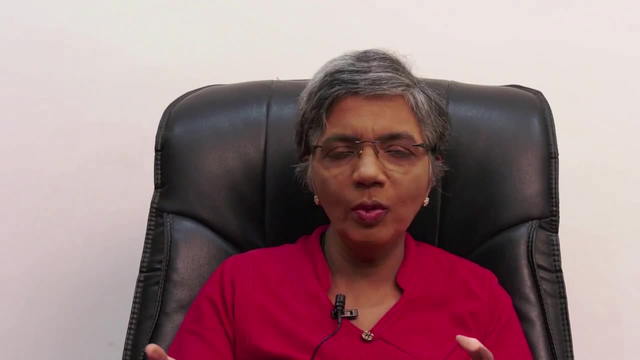 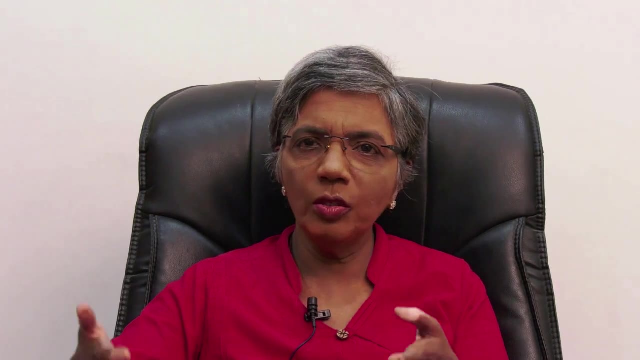